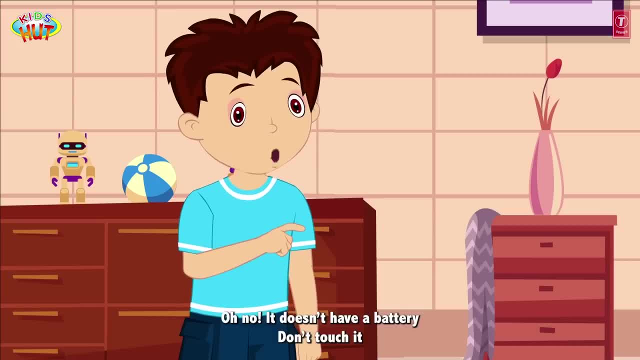 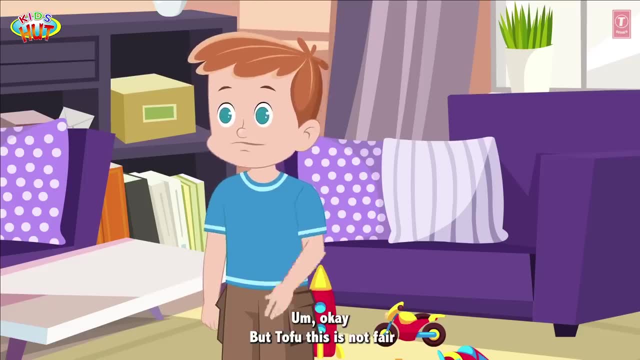 Can I play with it? Oh no, It doesn't have a battery. Don't touch it. Hmm, okay, But Tofu, this is not fair. I will not talk to you. Why aren't you not letting me play with your toys? 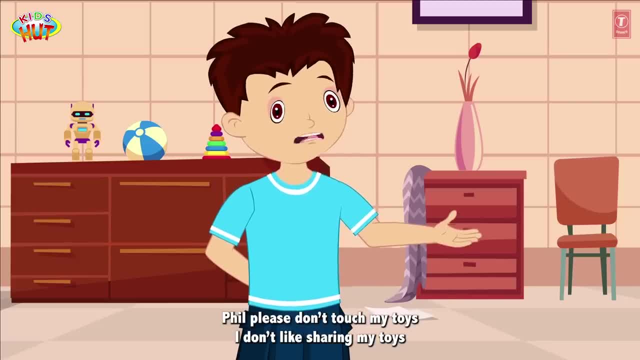 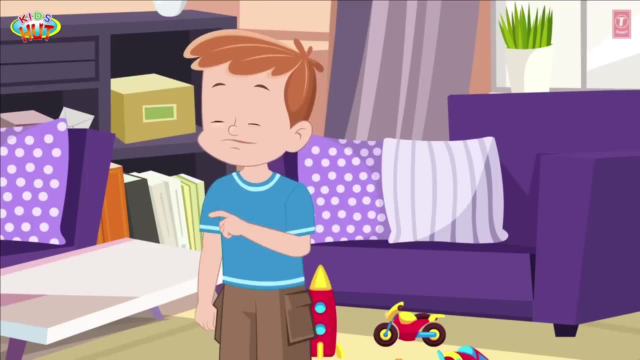 You are my friend, Phil. please Don't touch my toys. I don't like sharing my toys. Okay, Tofu, So I am going home. This is not what friends do. My mother told me good friends always share. 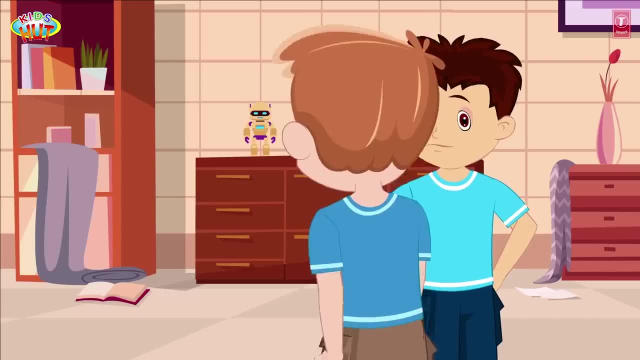 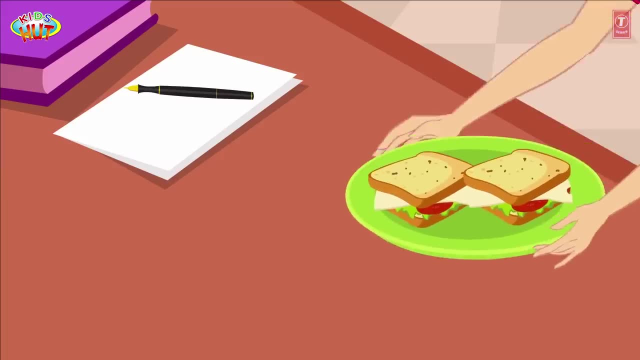 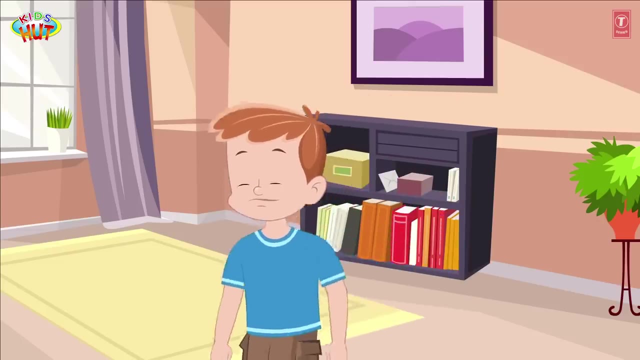 You are not a good friend. Bye, Tofu, Hmm, bye Phil. Wait, Phil, Don't be upset. I will talk to Tofu. He is a very good boy, Hmm, okay, Tia Tofu, say sorry to Phil and let him play with your toys. 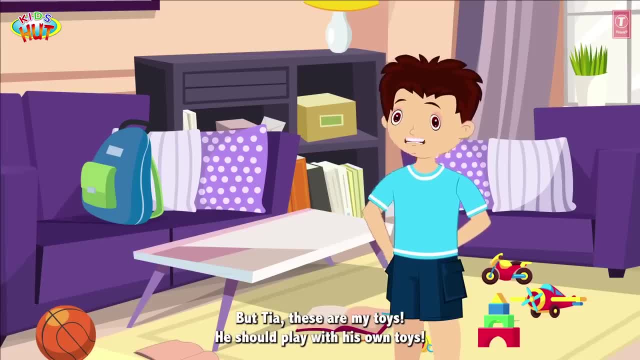 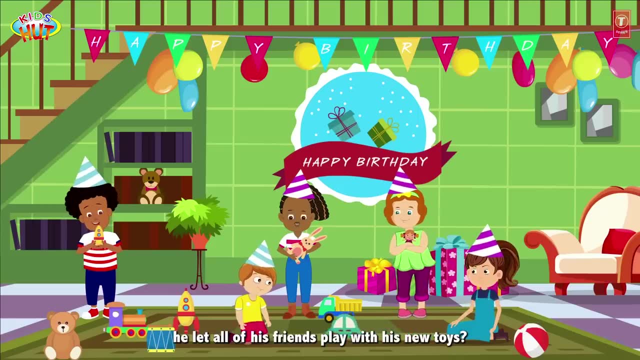 But, Tia, these are my toys. He should play with his own toys. Tofu, do you remember when you went to Phil's birthday party? He let all of his friends play with his new toys. You played with his toys too. 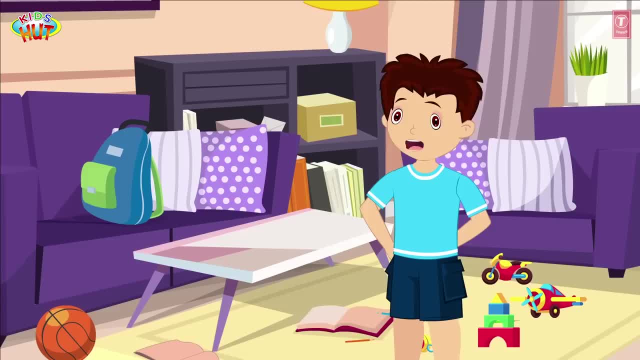 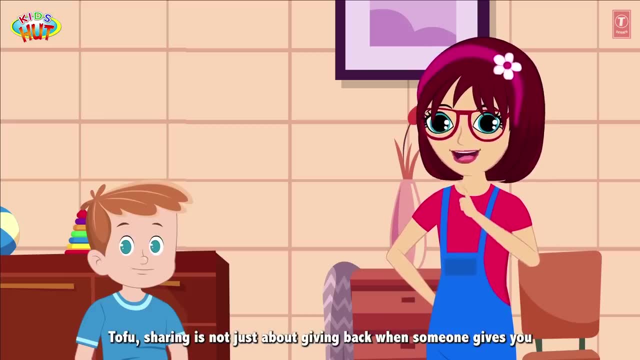 And Phil was so happy sharing his toys with everyone. Ah, yes, I remember Tofu. sharing is not just about giving back when someone gives you. It's about sharing to show that you care for them, no matter what, You should always be kind to everybody. 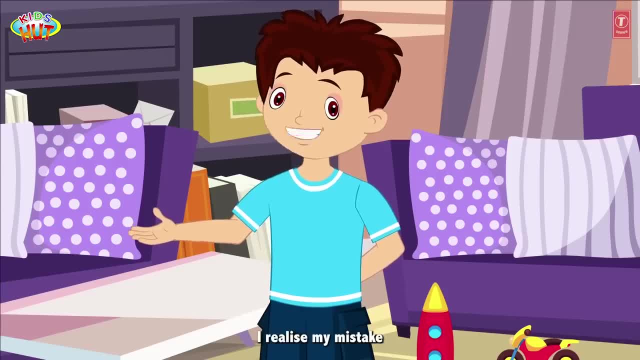 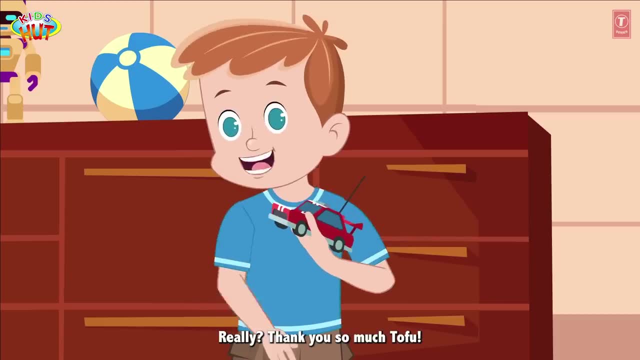 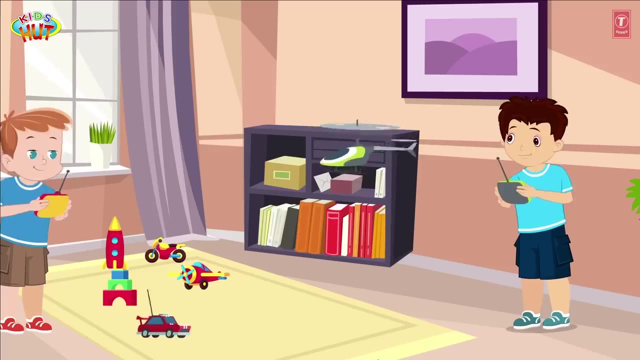 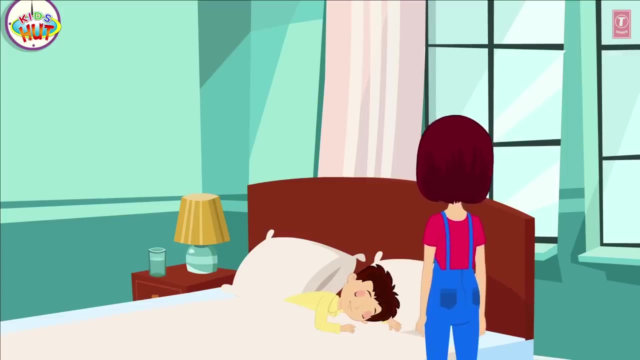 You are right, Tia. I am sorry, Phil, I realised my mistake. You can play with my toys Really. Thank you so much, Tofu. Thank you, Tia, You are welcome. Phil. Tofu, wake up, It's time to go to school. 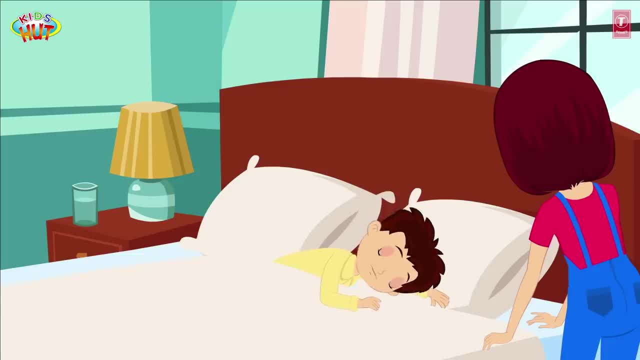 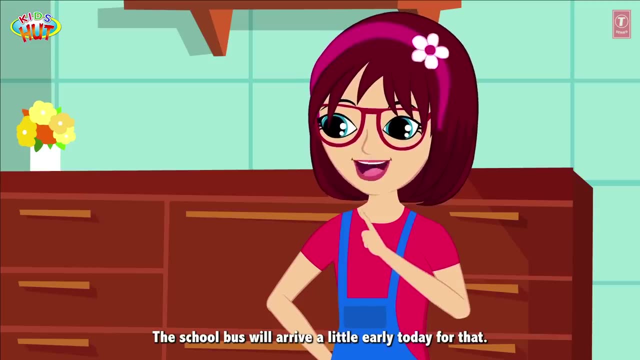 But Tia, the school bus arrives at 8 am. Tofu, don't you remember? You have to go to a school picnic today. The school bus will arrive a little early today for that School picnic. Oh yes, I forgot about it. 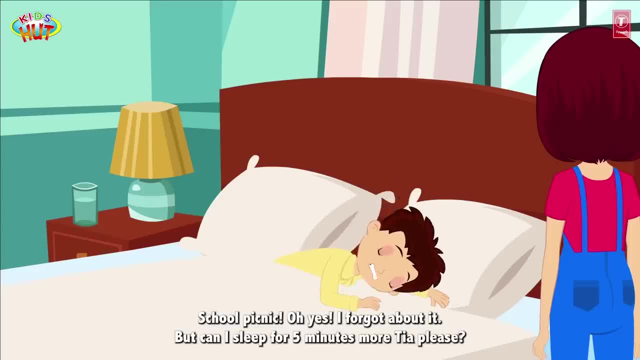 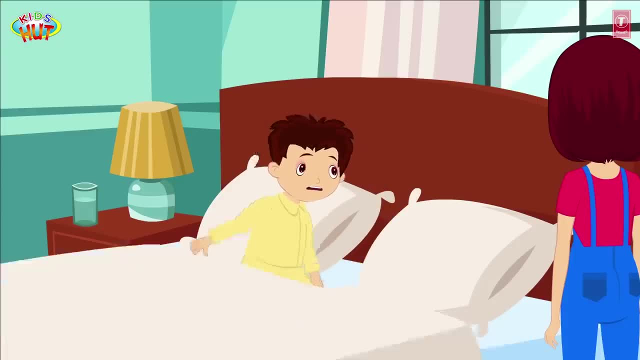 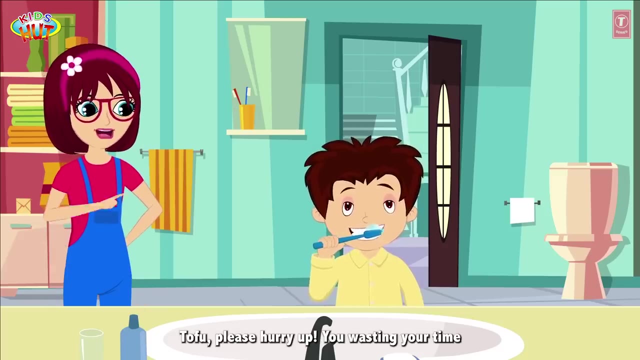 But can I sleep for five minutes more? Tia, please, You will miss the bus. Tofu, Come on, get up. Okay, Tofu, please, hurry up. You are wasting your time. You will not be able to make it to the school picnic otherwise. 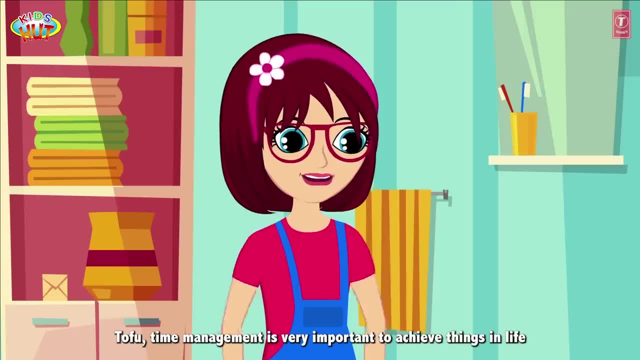 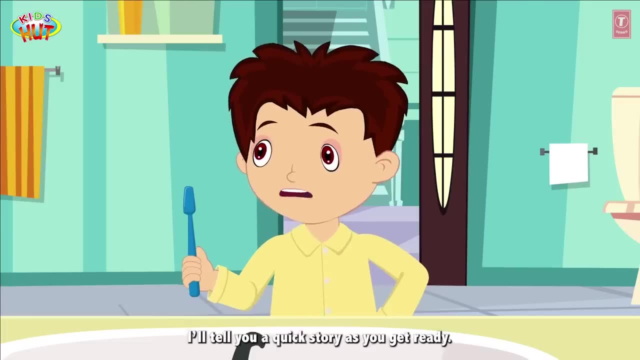 I still have half an hour to catch the bus. Tia Tofu. time management is very important to achieve things in life. Now, what does that mean, Tia? I'll tell you a quick story as you get ready, Okay. 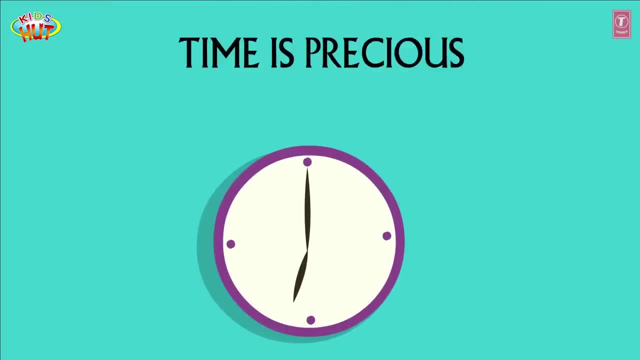 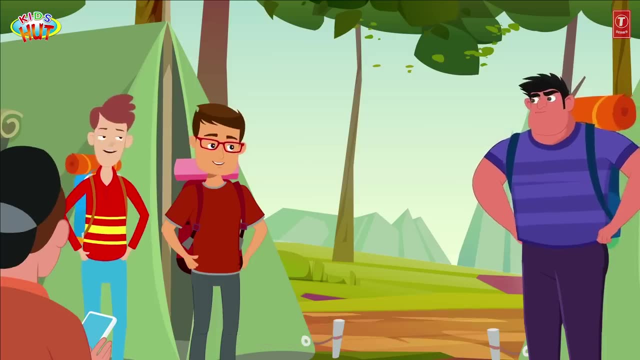 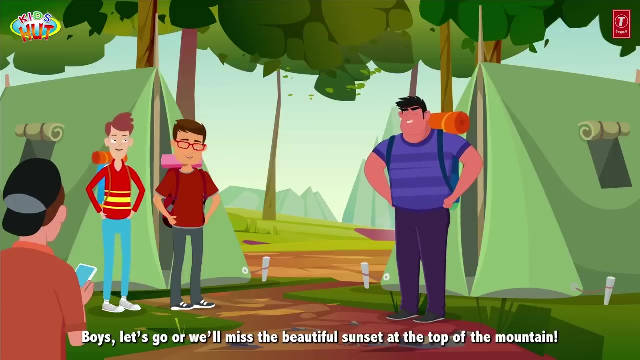 Time is precious. Once upon a time, a boy named Oliver went for a hiking trip with a group of other people. Oliver wasted a lot of time, and hence he missed a lot of things. always, Boys, let's go, Or we'll miss the beautiful sunset at the top of the mountain. 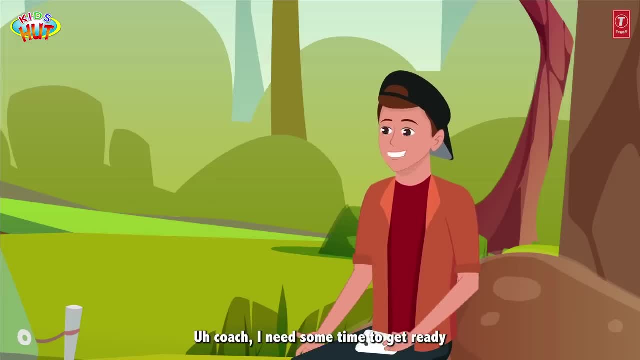 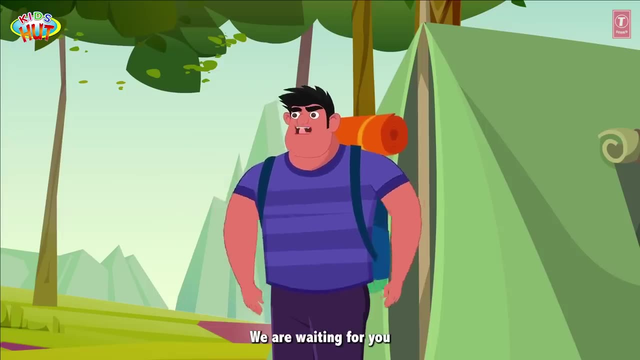 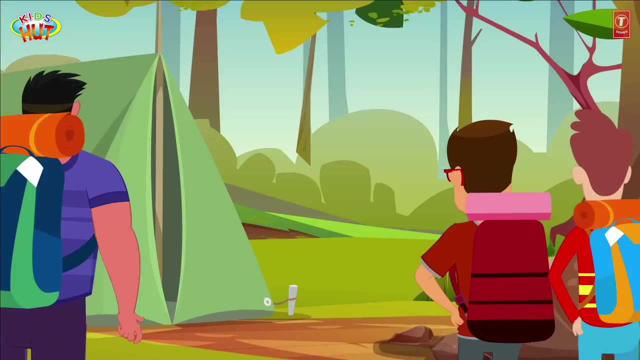 Yes, sir, Let's go. Coach, I need some time to get ready. You should have been ready by now. Oliver, Come back fast. We're waiting for you. Yes, sir, Oliver, please hurry up. You're wasting your time and everybody else's time too. 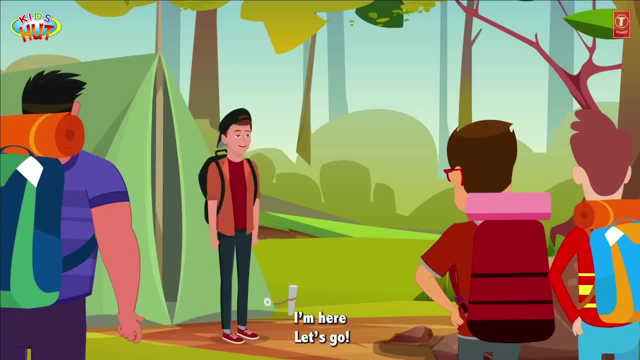 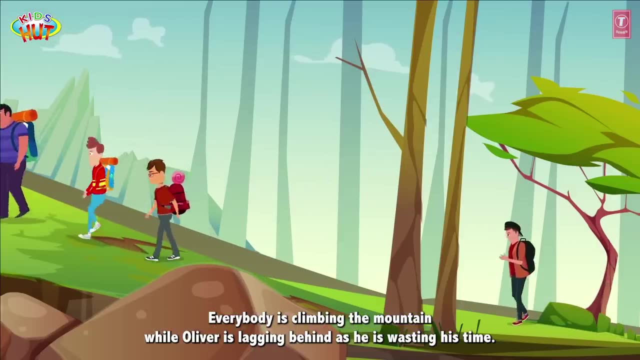 We can't wait for you anymore. I'm here, Let's go. Everybody is climbing the mountain, while Oliver is lagging behind as he is wasting his time. Where is Oliver? I can't see him. Coach, he is resting there. 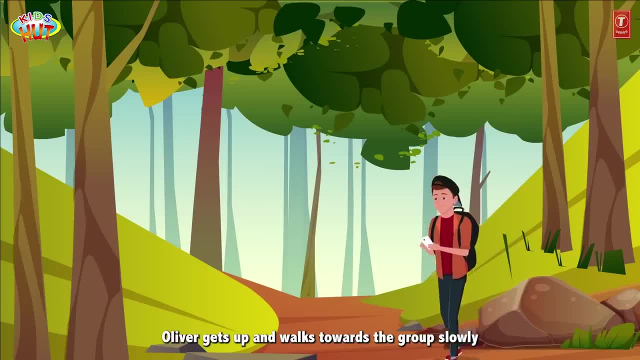 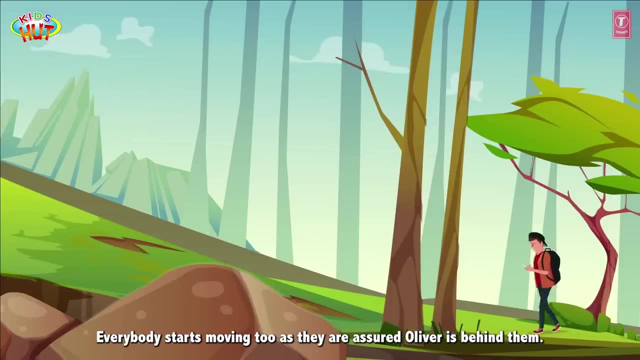 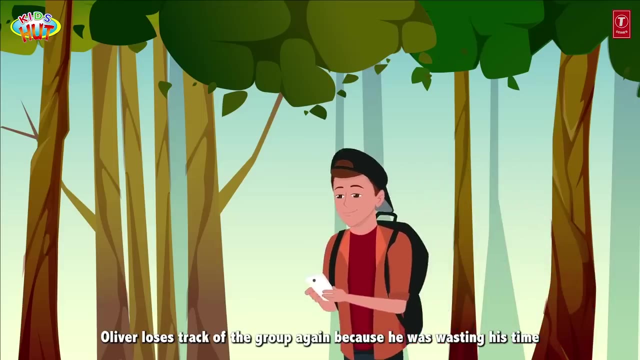 Oliver, hurry up. Oliver gets up and walks towards the group. slowly. Everybody starts moving too, as they are assured Oliver is behind them. As everybody is climbing the mountain, Oliver loses track of the group again because he was wasting his time. He starts panicking as he was lost. 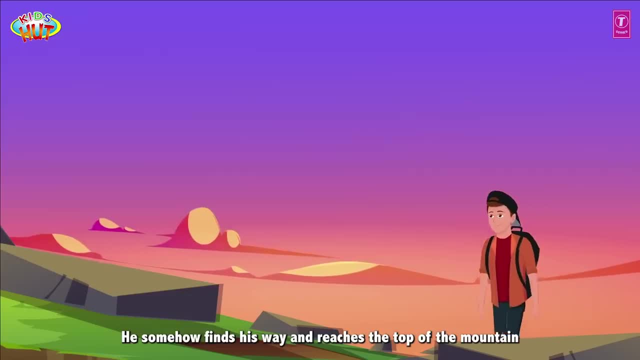 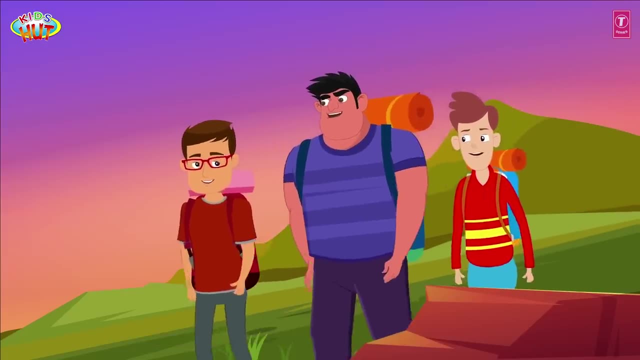 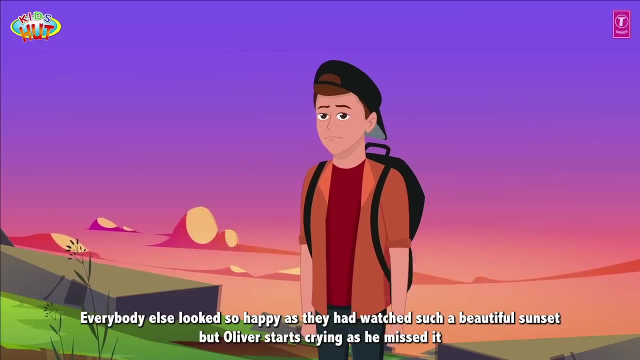 He somehow finds his way and reaches the top of the mountain, But when he reaches, the sun had already set and everybody was walking down the mountain. Everybody else looked so happy as they had watched such a beautiful sunset, But Oliver starts crying as he missed it. 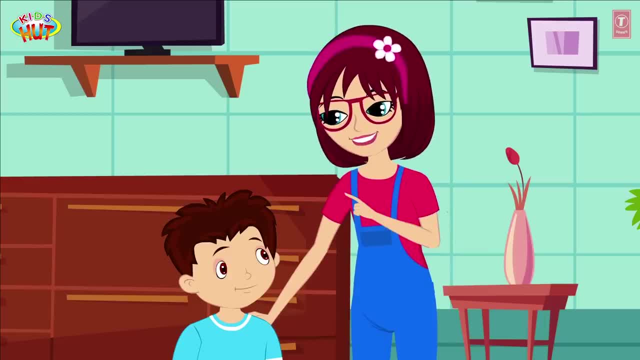 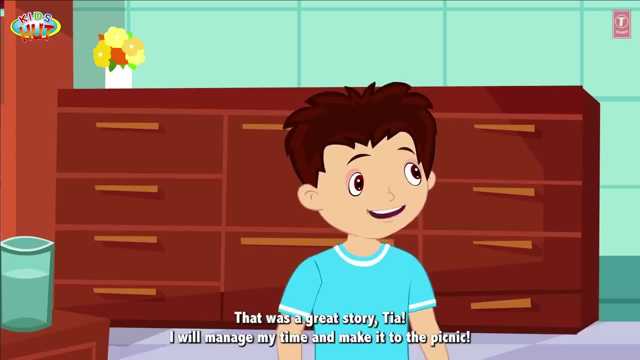 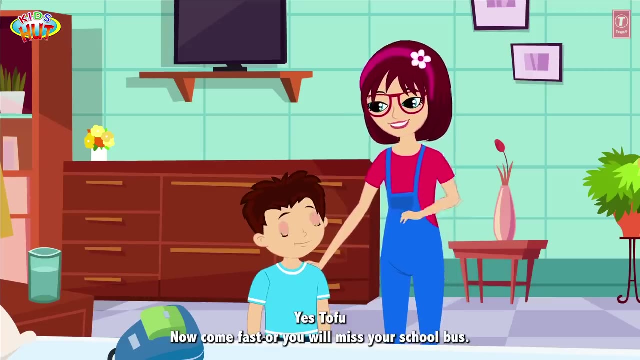 Time is precious. It waits for no one. Once you start managing your time correctly, you will achieve a lot of beautiful things in life. That was a great story, Tia. I will manage my time and make it to the picnic. Yes, Tofu. Now come fast or you will miss your school bus. 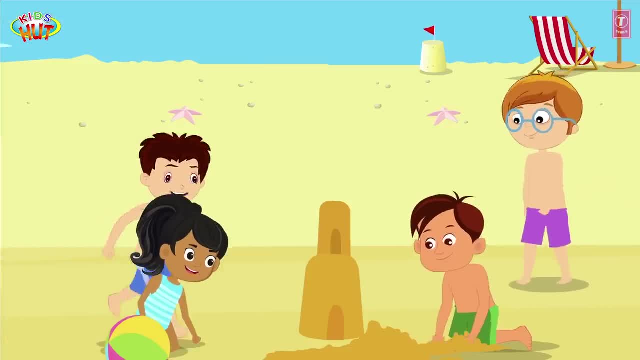 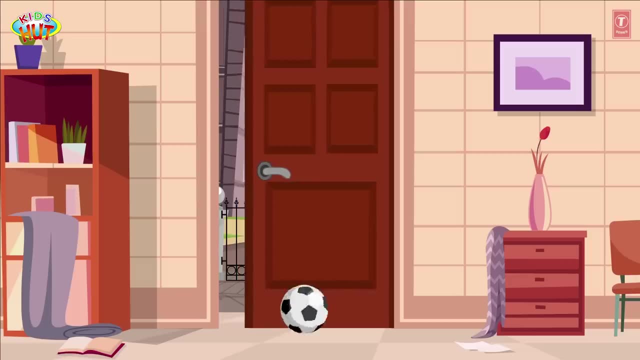 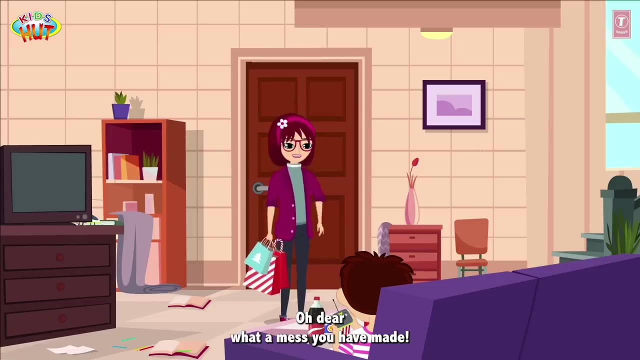 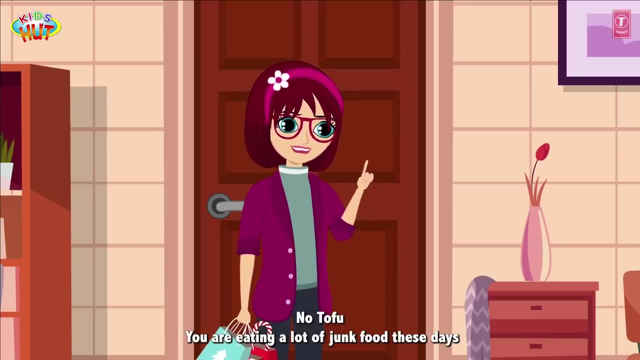 Ok, Oh dear, what a mess you have made. Hi, Tia, Did you get me some chips and chocolates? No Tofu. You are eating a lot of junk food these days, But, Tia, I don't like eating vegetables and fruits. 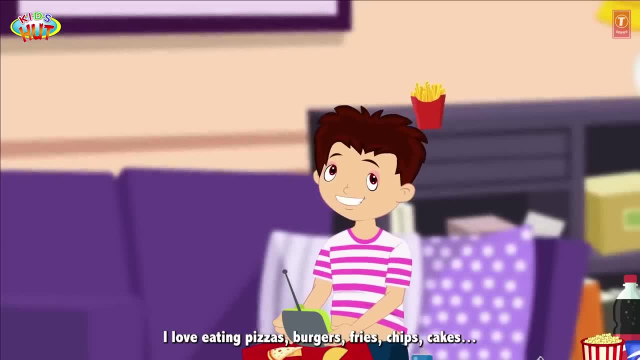 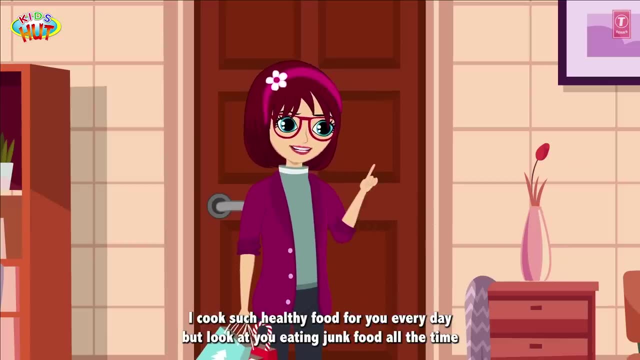 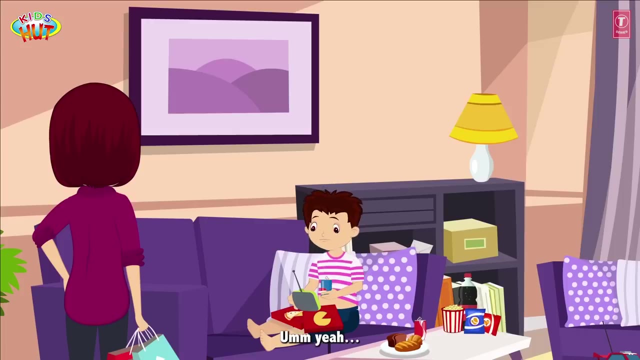 I love eating pizzas, burgers, fries, chips, cakes. I cook such healthy food for you every day, But look at you eating junk food all the time. It's so harmful for the body and your health. Hmm, Yeah, Tofu. clean this mess and complete your homework. 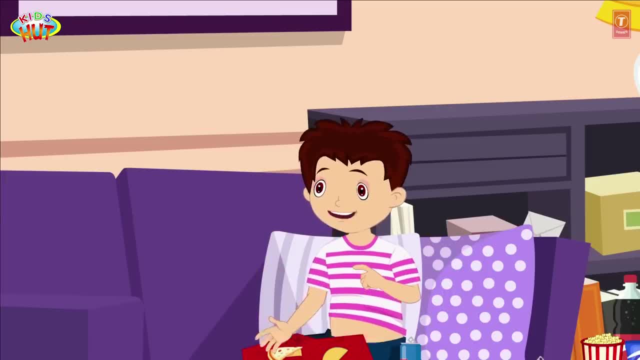 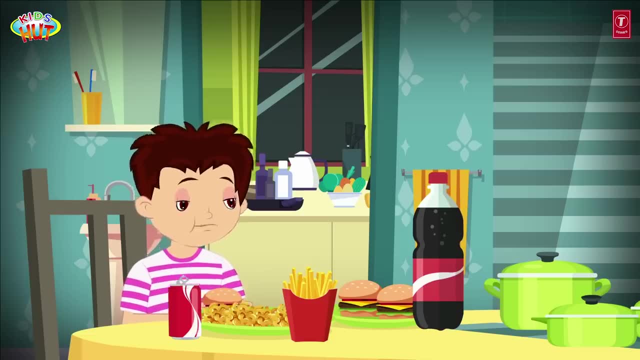 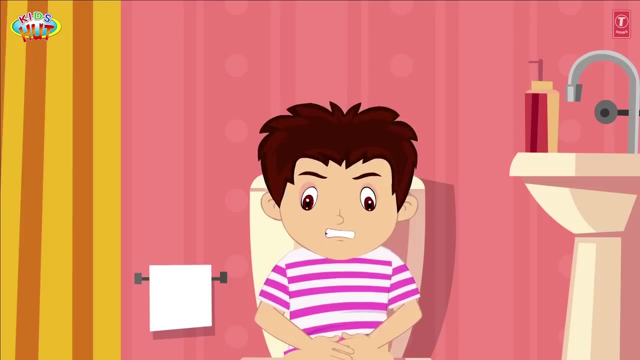 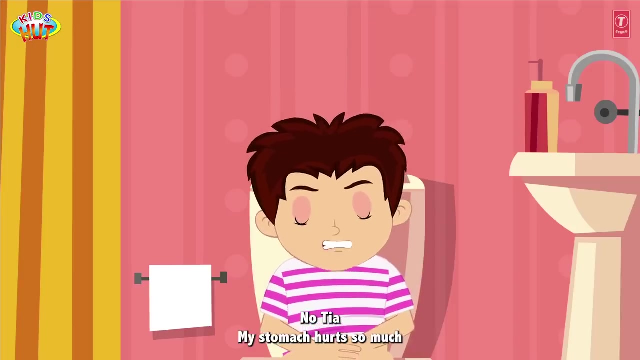 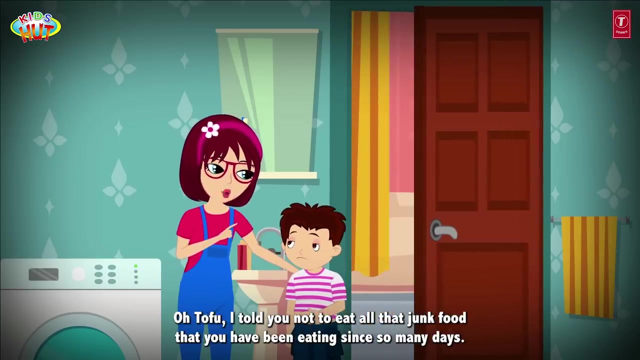 I will. I will, Tia, Don't worry. Tofu is everything alright? No, Tia, My stomach hurts so much. I feel sick. Oh, Tofu, I told you not to eat all that junk food that you have been eating since so many days. 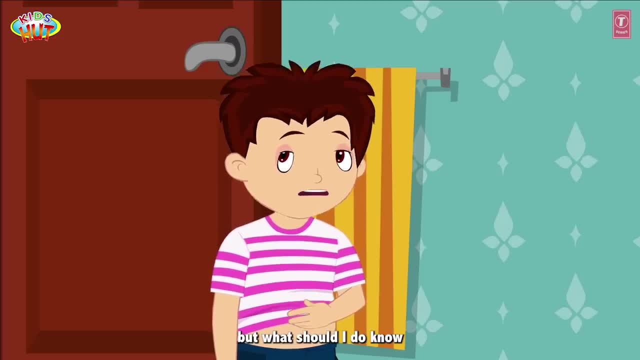 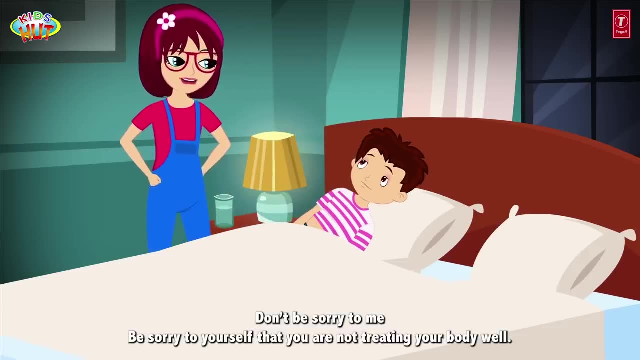 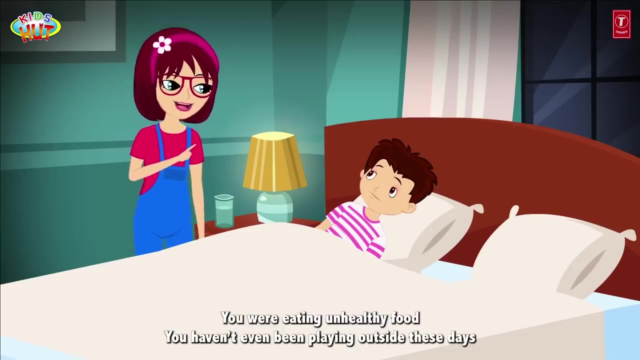 I am sorry, Tia, But what should I do now? Don't be sorry to me. Be sorry to yourself that you are not treating your body well, Tia, but how did I feel sick? because of food. You were eating unhealthy food. You haven't even been playing outside these days. 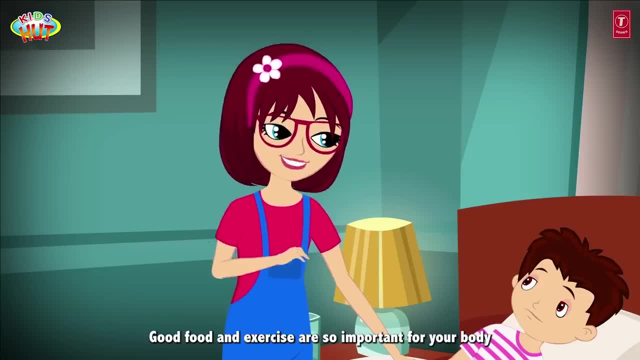 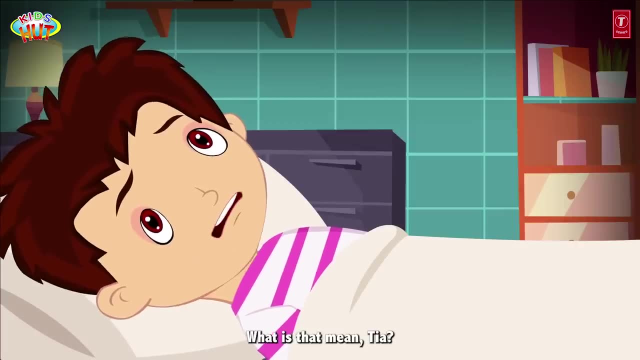 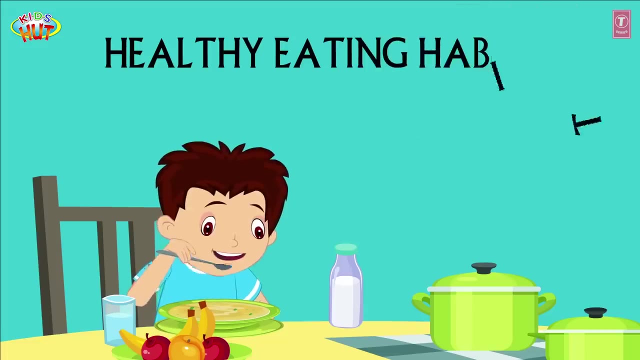 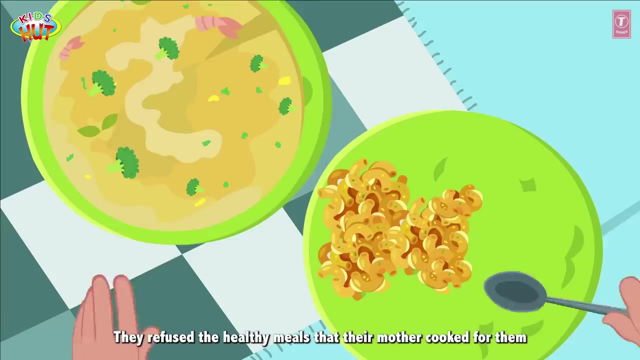 Good food and exercise are so important for your body. Remember what you eat is what you become. What does that mean? Tia? Healthy Eating Habits. Once upon a time, there lived two siblings who loved eating junk food. every day, They refused the healthy meals that their mother cooked for them. 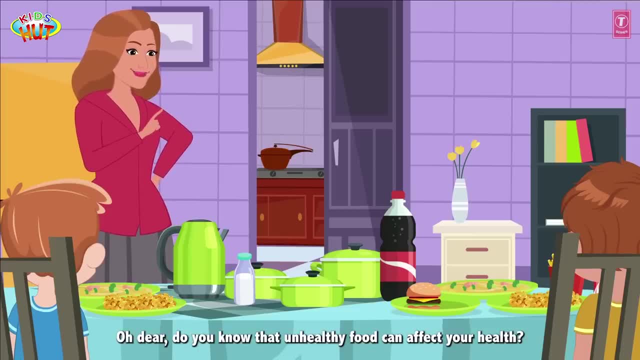 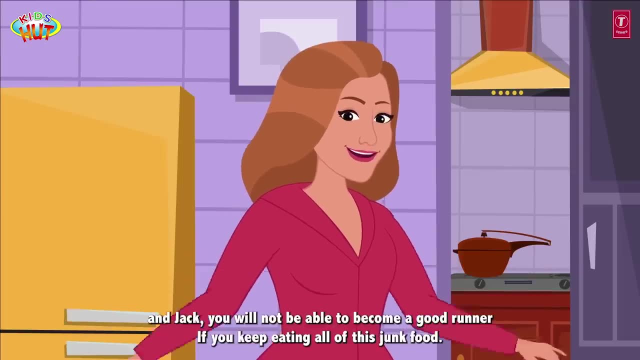 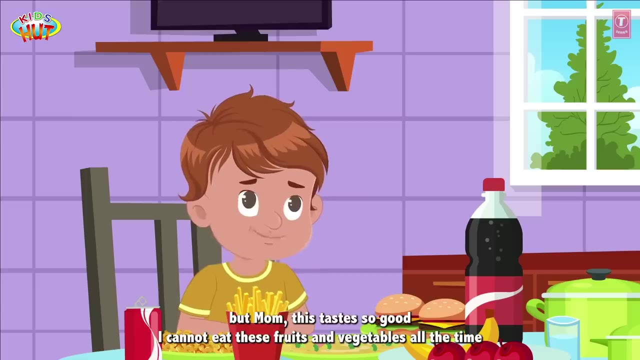 Oh dear. Do you know that unhealthy food can affect your health? Joe, you will not be able to play football so well And, Jack, you will not be able to become a good runner if you keep eating all of this junk food. But, mom, this tastes so good. I cannot eat these fruits and vegetables all the time. 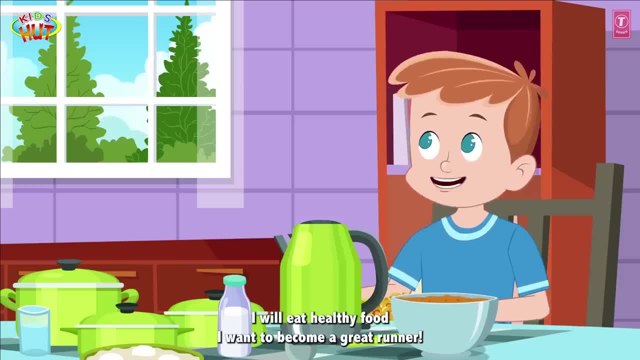 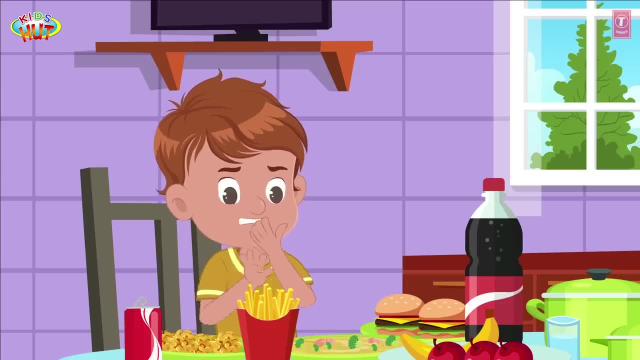 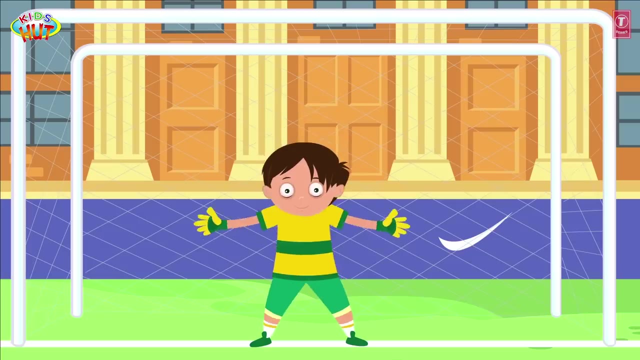 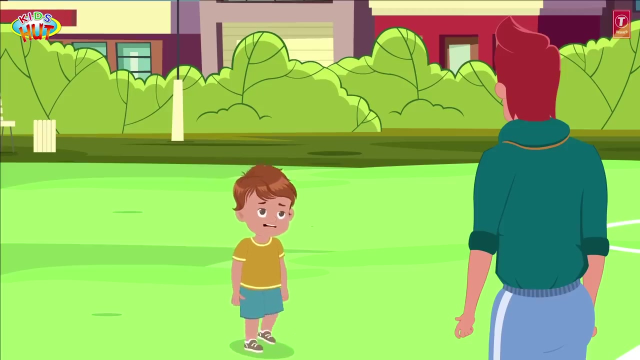 I will eat healthy food. I want to become a great runner. Yes, Jack, Eat healthy and you will see the difference. Joe, you too, Joe, come here. I am sorry, but I cannot have you on the team. You are not able to play like others. 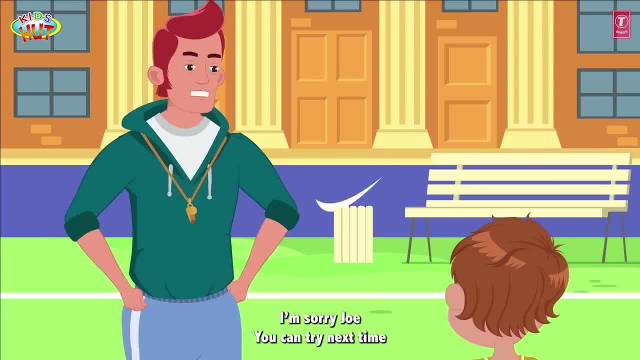 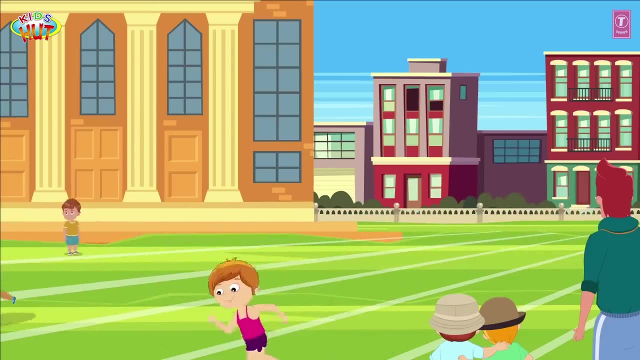 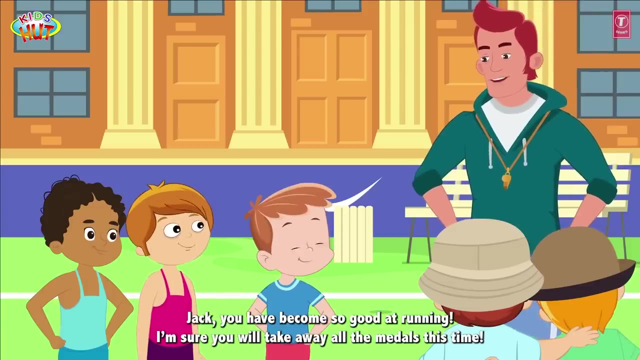 But, coach, I want to be on the team. I am sorry, Joe. You can try next time. Jack, you have become so good at running, I am sure you will take away all the medals this time. Thank you, coach. 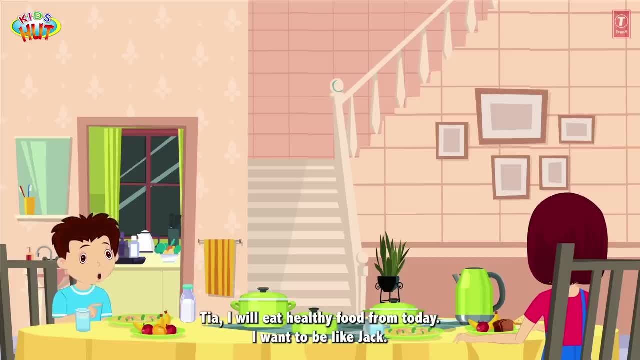 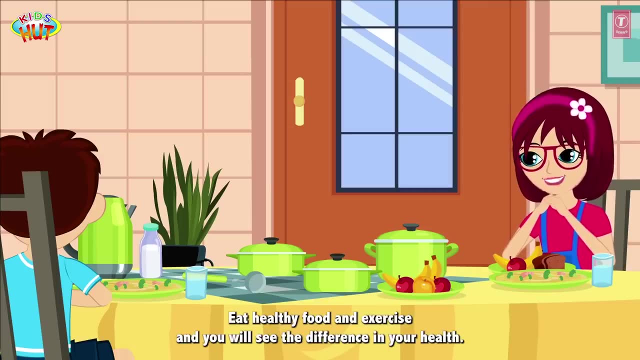 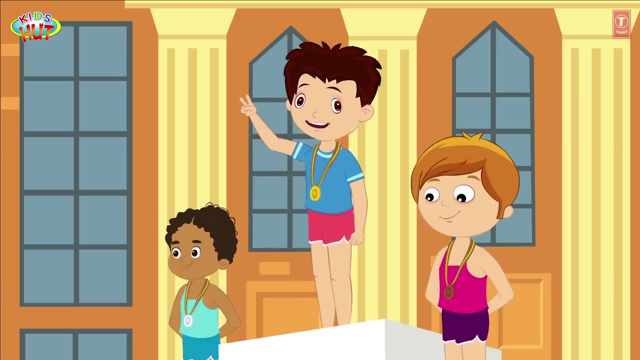 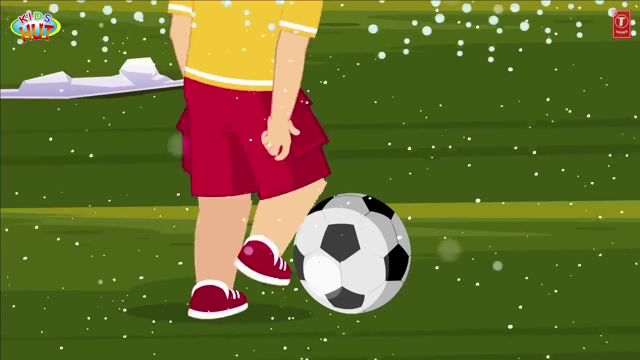 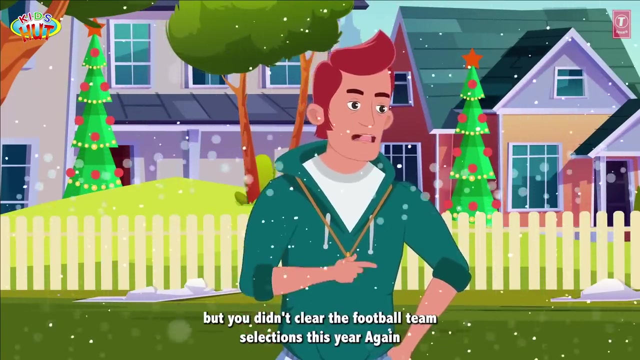 Tia, I will eat healthy food from today. I want to be like Jack. Yes, Tofu, Eat healthy food and exercise and you will see the difference in your health. Tofu, I am sorry but you didn't clear the football team selections this year again. 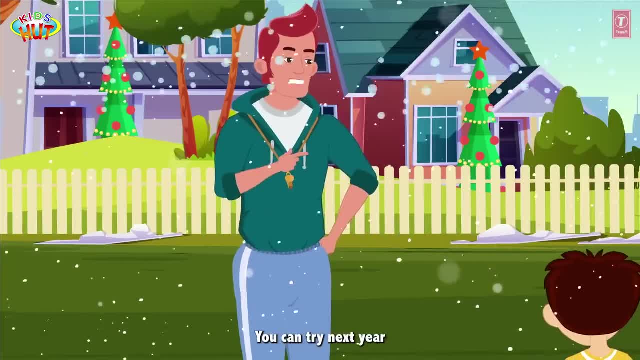 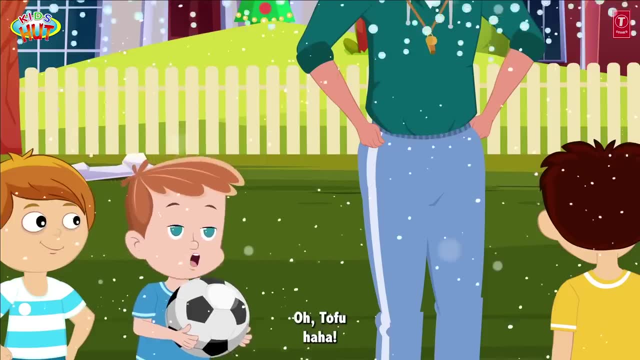 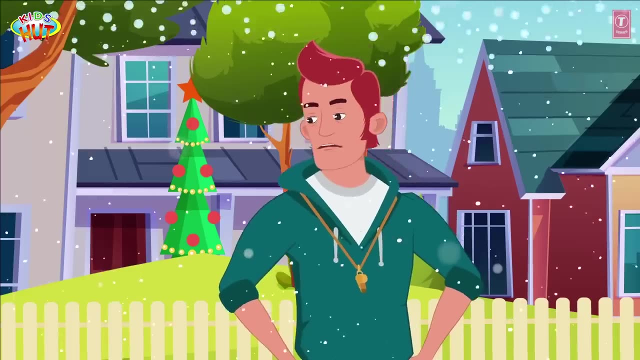 You can try next year, But, coach, give me a chance please. I promise I will do my best. Oh Tofu, Haha, I bet you won't be able to clear the selections next year too. Joe, stop being mean, or I won't select you either. 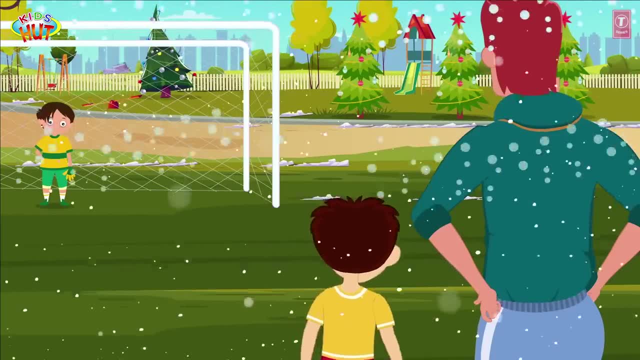 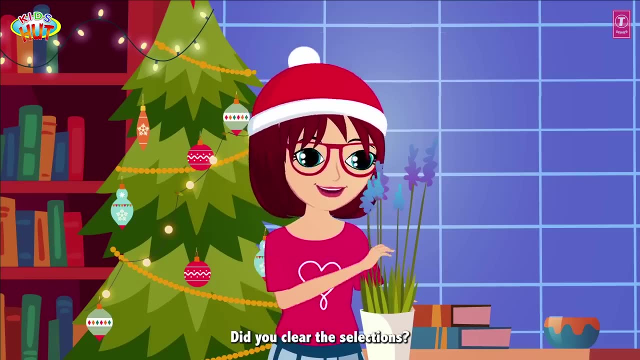 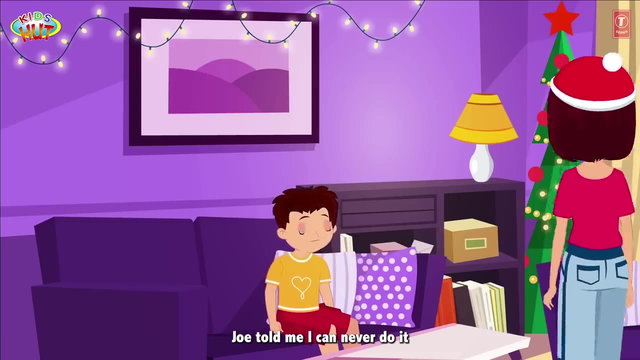 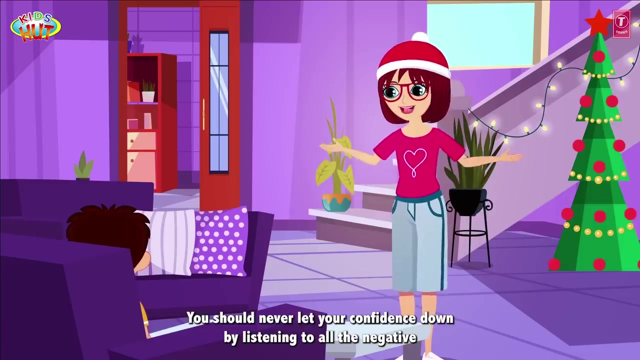 I am sorry, coach, What's up? Did you clear the selections? No, Tia, I didn't clear it this year too. Joe told me I can never do it. Let people talk. You should never let your confidence down by listening to all the negative things that people say to you. 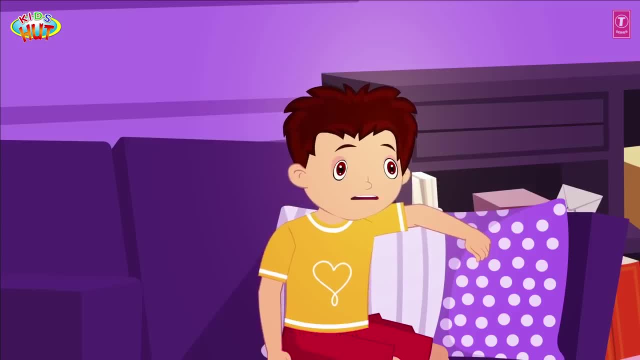 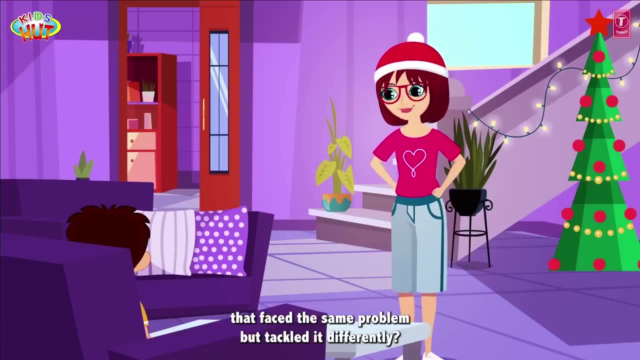 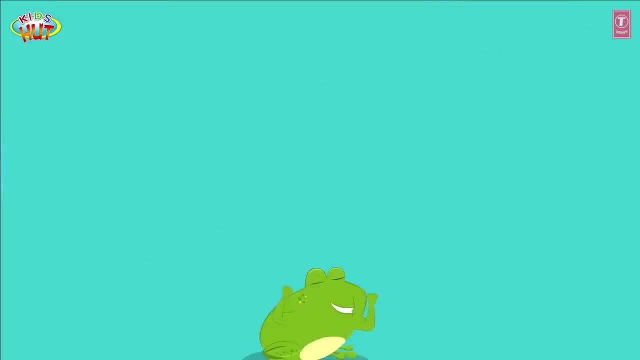 I feel terrible. Tia, I can never get in. I tried so hard this year. Tofu, you want to hear a story about two frogs that faced the same problem but tackled it differently? Yes, please Never Stop Believing. 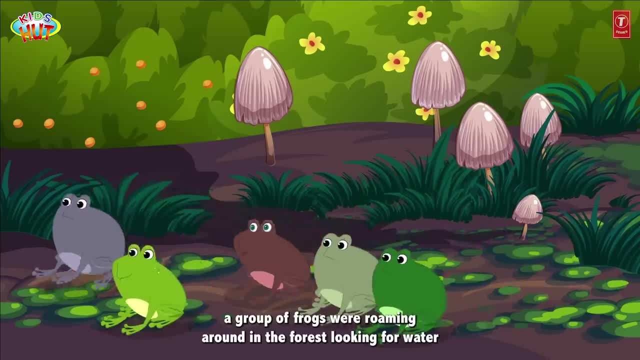 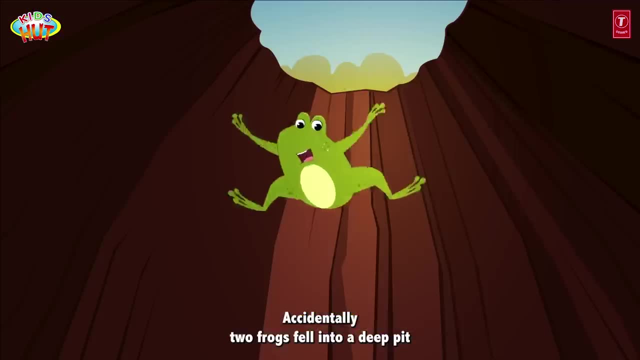 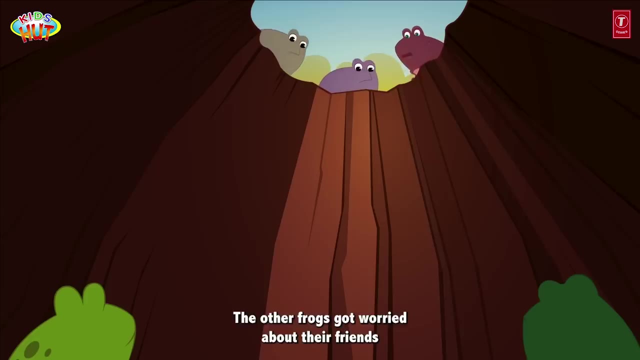 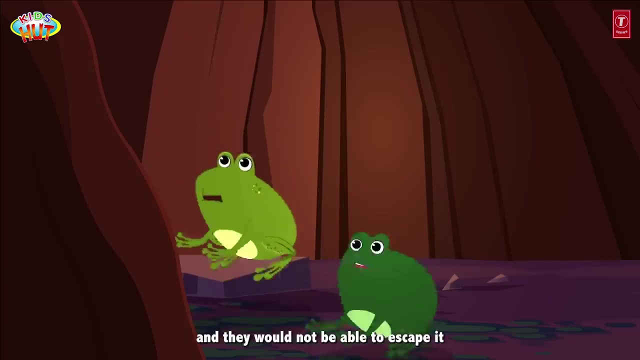 Not so long ago, a group of frogs were roaming around in the forest looking for water. Accidentally, two frogs fell into a deep pit. They were terrified to death about whatever just happened. The other frogs got worried about their friends. They thought that the pit was too deep and they would not be able to escape it. 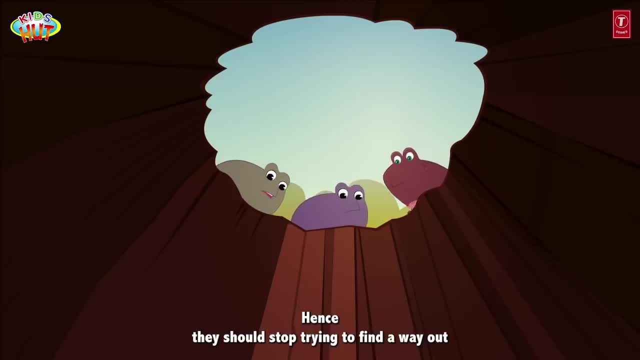 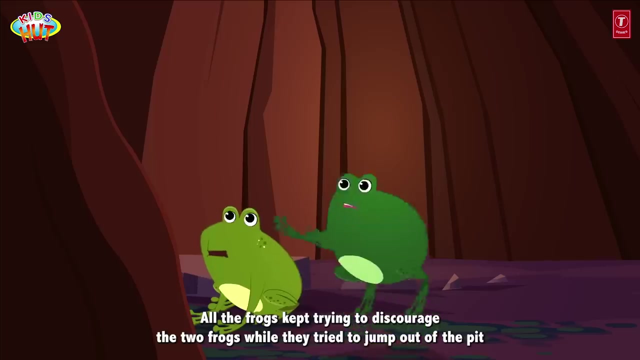 Hence they should stop trying to find a way out. You will never be able to come out of the pit. It's too deep. It looks impossible, my dear friends, What do we do now? All the frogs kept trying to discourage the two frogs while they tried to jump out of the pit. 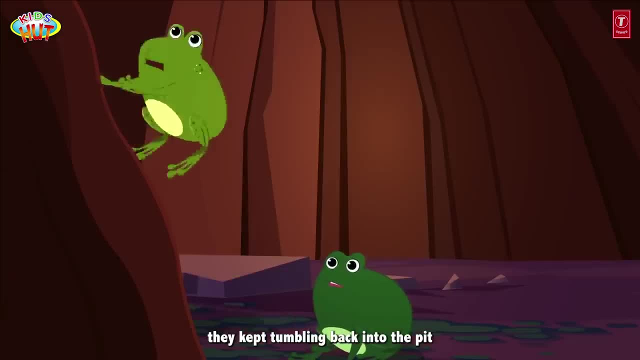 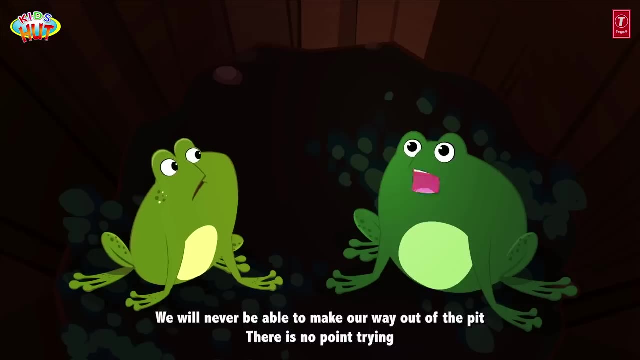 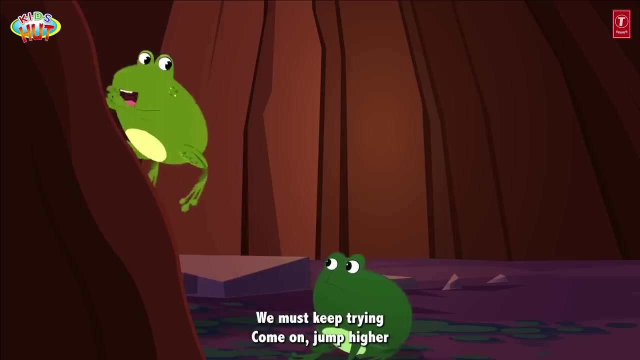 Despite all the effort, they kept tumbling back into the pit. Oh, my dear friends, you were right. We will never be able to make our way out of the pit. There is no point trying. We must keep trying. Come on, jump higher, We can do it. 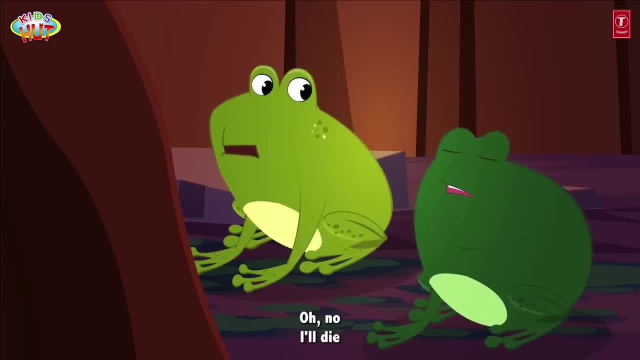 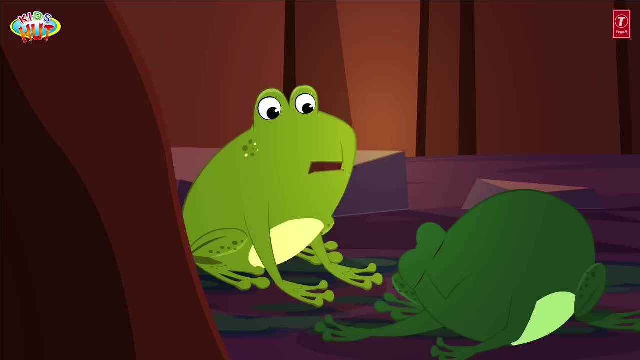 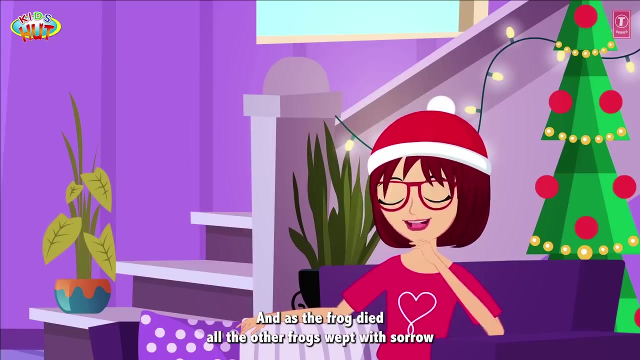 I'll die. Oh no, I'll die. And as the discouraged frog said these words, he died on the spot. Oh no, my friend, You gave up too soon. And as the frog died, all the other frogs wept with sorrow. 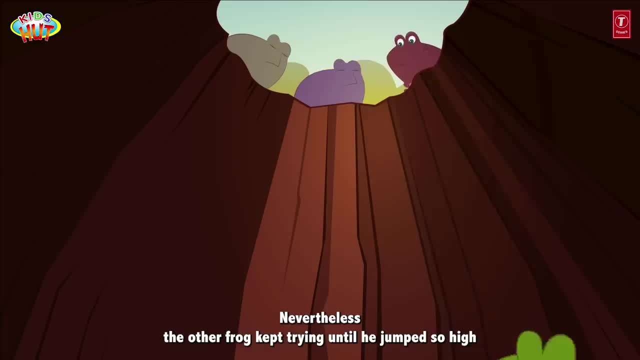 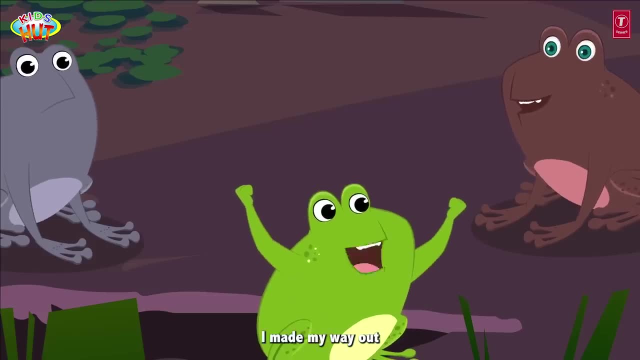 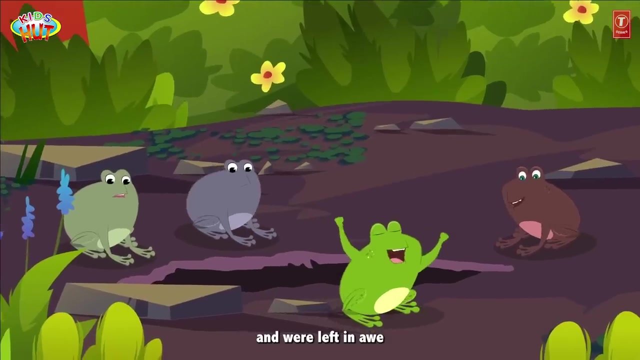 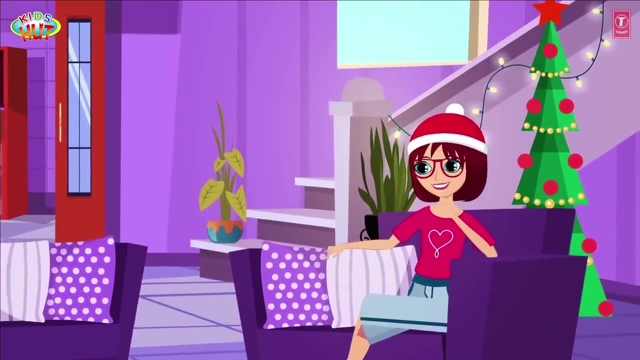 Nevertheless, the other frogs kept trying. He kept trying until he jumped so high that he escaped the pit. I made it. I made my way out. All the other frogs were shocked at what just happened and were left in awe. To everybody's surprise, the other frog turned out to be deaf, and hence he couldn't hear the discouragement thrown at him. 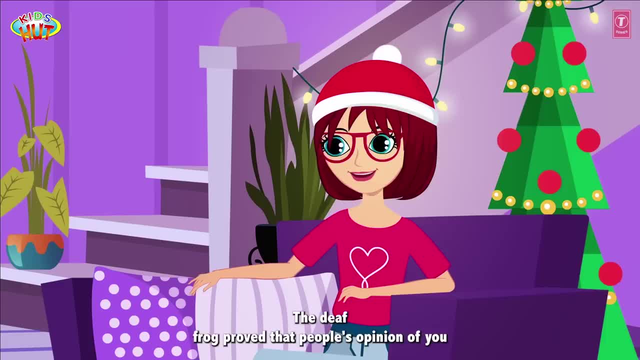 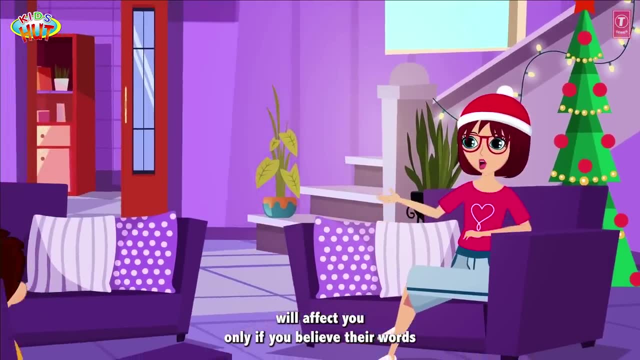 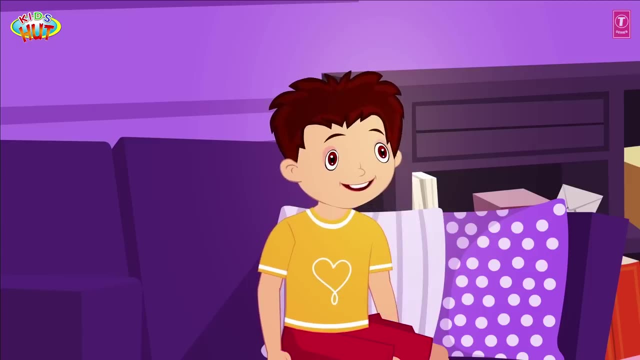 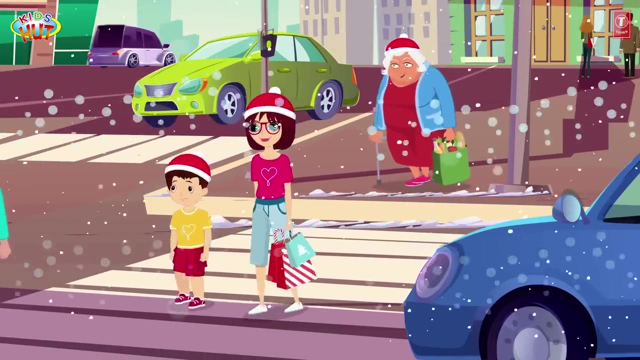 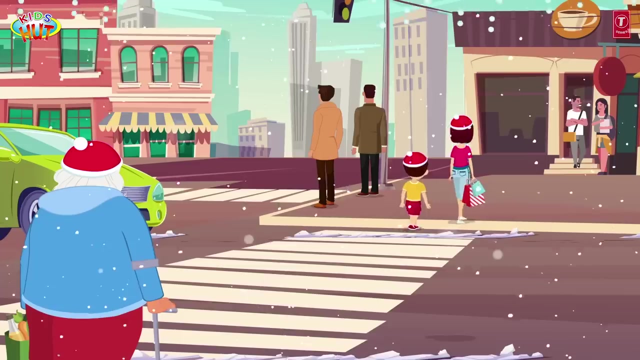 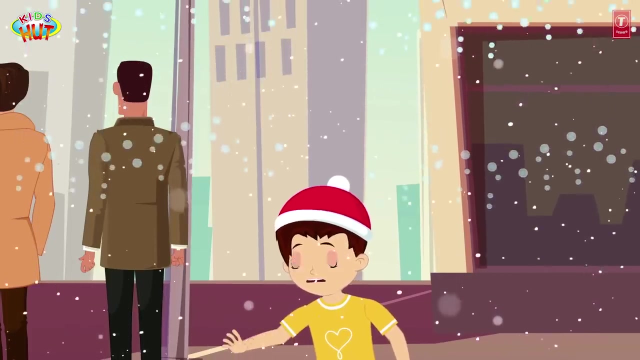 He thought his friends were cheering him on. The deaf frog proved that people's opinion of you will affect you only if you believe their words. rather than believing in yourself and being confident, He is, now arises to believe in himself and his family. In an instant, the other frog says something. 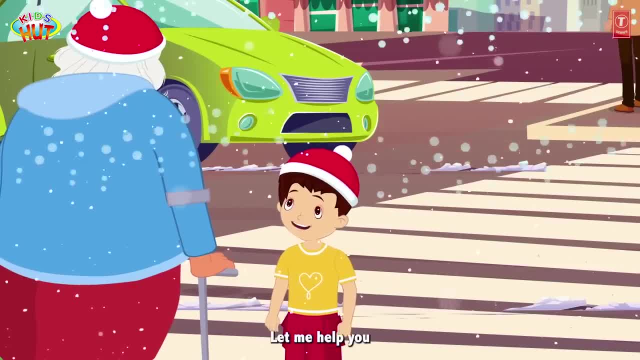 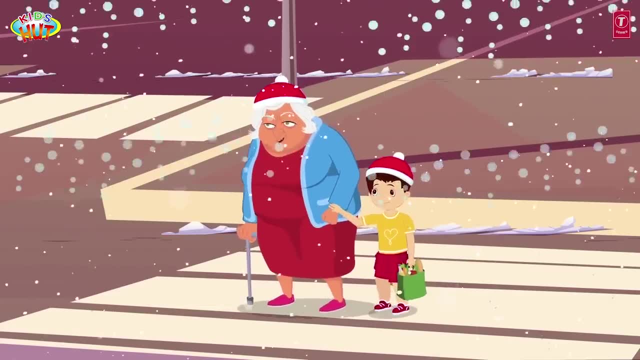 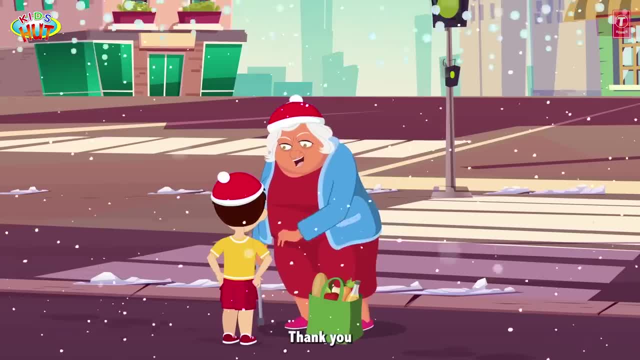 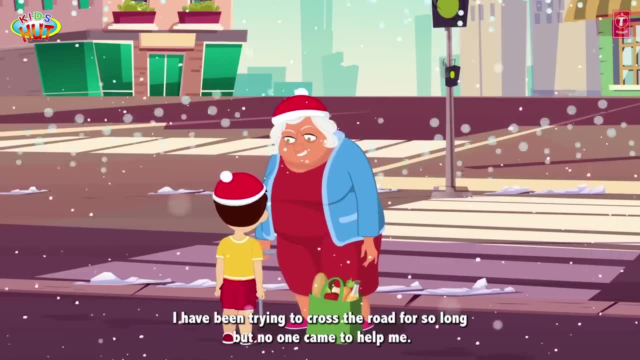 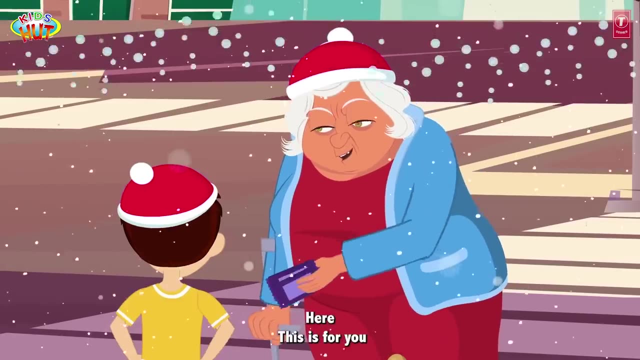 I'm back. Hello, Miss, let me help you. I'm going to help you, Kind of you. I have been trying to cross the road for so long, but no one came to help me. It's my pleasure, Miss, Here. this is for you. 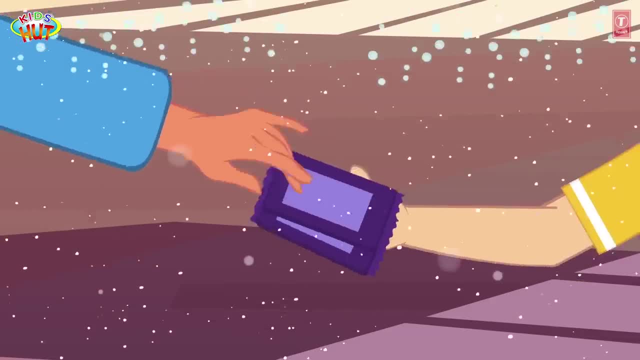 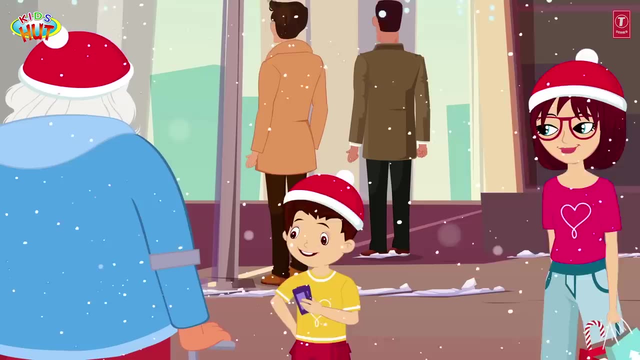 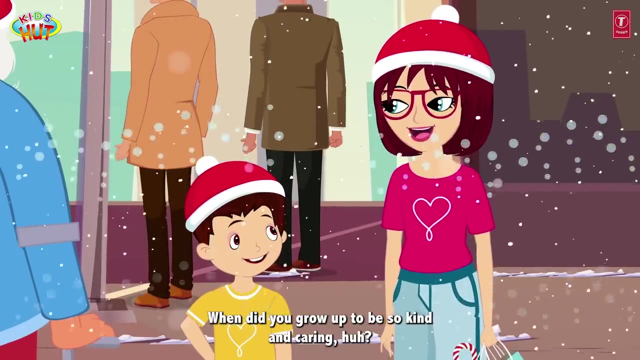 You have been really kind to me. Oh, Chocolates, Thank you so much. Wow, Tofu, I am so proud of you. When did you grow up to be so kind and caring? huh, You remind me of a beautiful story. 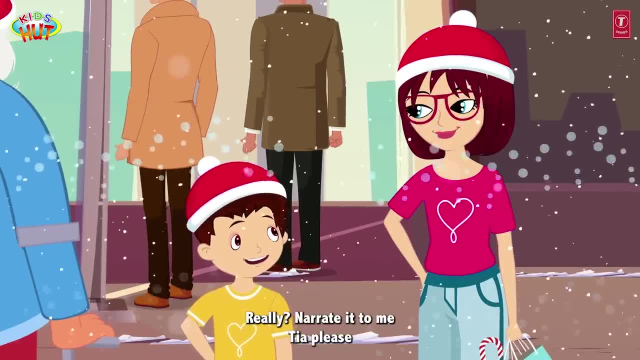 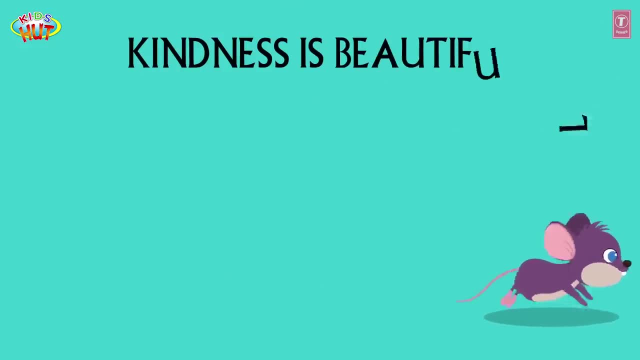 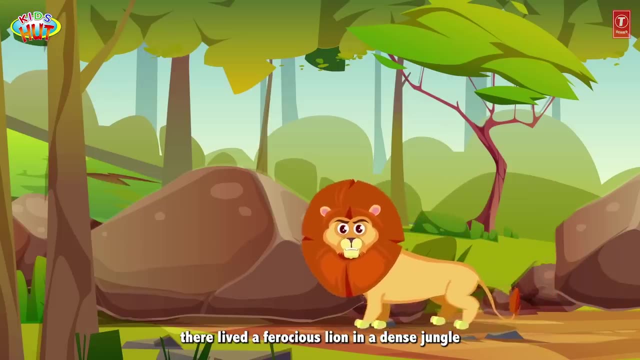 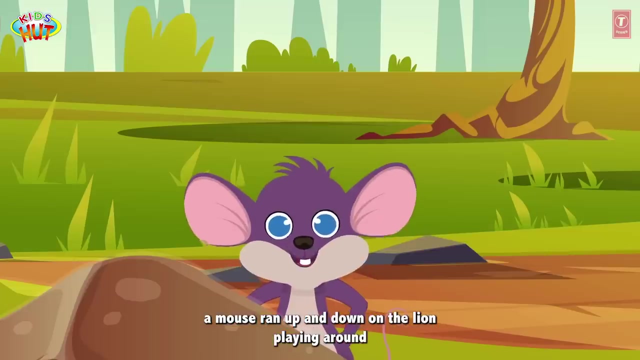 Really Narrate it to me, Tia, Please. Kindness is beautiful. Once upon a time there lived a ferocious lion in a dense jungle. One day, when the lion was asleep under the cool shade of a tree, a mouse ran up and down on the lion. 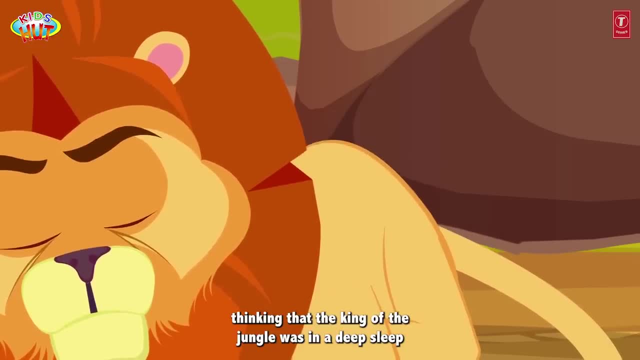 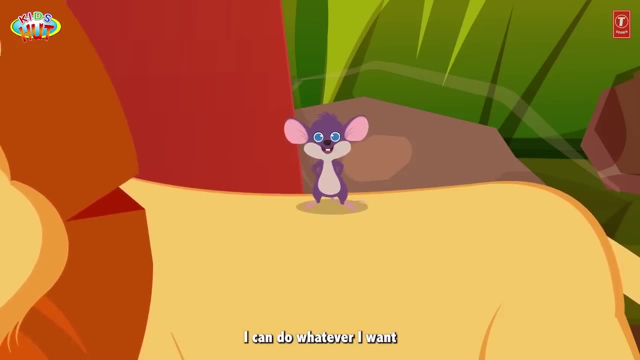 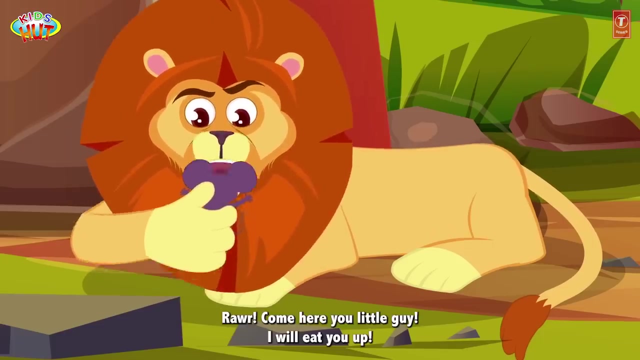 playing around thinking that the king of the jungle was in a deep sleep. Whee, The king is asleep. I can do whatever I want. Come here, you little guy, I will eat you up. Oh no, Please leave me, sir.